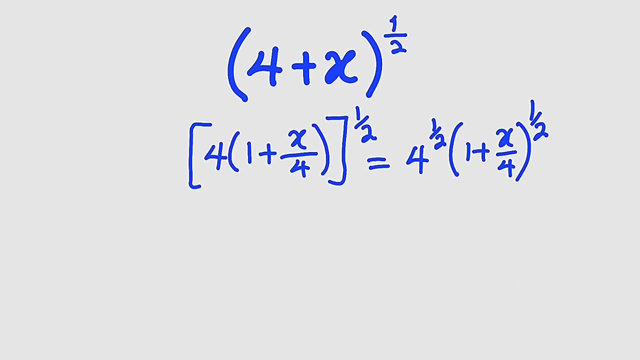 You know that 4 to the power of 1 divided by 2 is the same thing as square root of 4, which is equal to 2.. So this is equal to 2 multiplied by 1 plus x divided by 4, all to the power of 1 divided by 2.. 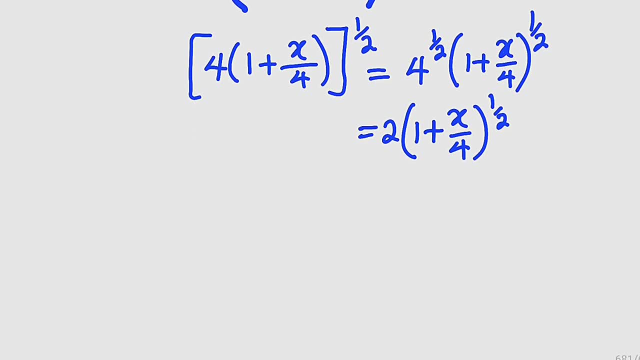 Alright, let me take that term and expand it. That is 1 plus x divided by 4, raised to the power of 1 divided by 2, before we come back to that 2.. So what is our formula? Remember that our formula is 1 plus nb. 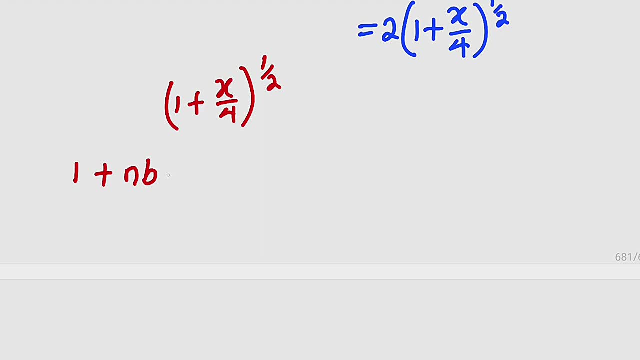 n is the power, b is this term. Then the third term will be n multiplied by n minus 1, then b squared, divided by 2 factorial. We are looking for the only 4 terms, so let me add one more. We have n multiplied by n minus 1, multiplied by n minus 2, then b raised to the power of 3, divided by 3 factorial. 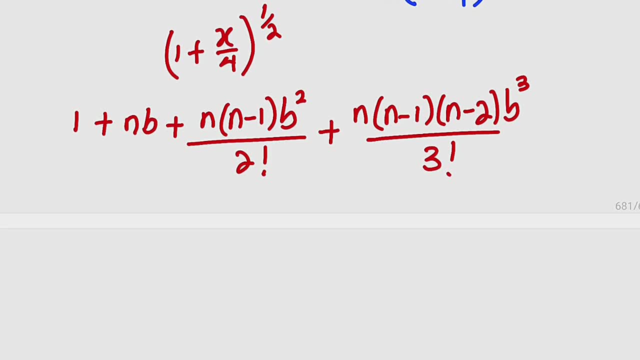 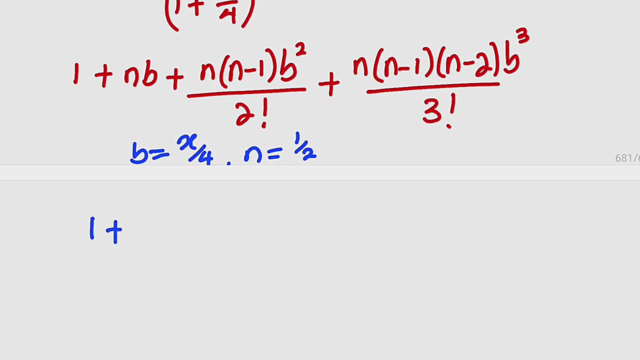 So now let us substitute this For which, For which I told you that b is equal to x divided by 4 and n is equal to 1 divided by 2.. So our first term will be 1.. Our second term will be nb. 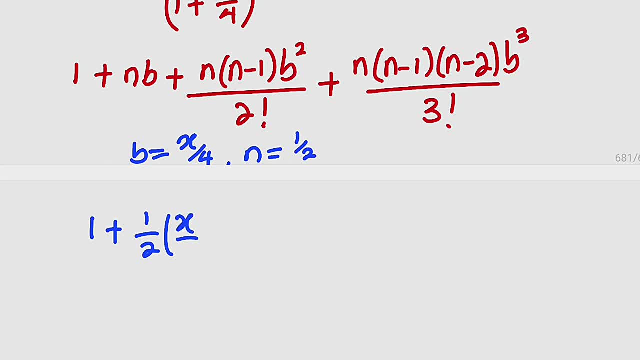 1 divided by 2 multiplied by x divided by 4.. This is our second term Plus n, which is 1 divided by 2, multiplied by 1.. 1 divided by 2 minus 1, then b squared, and b is x divided by 4, all squared right. 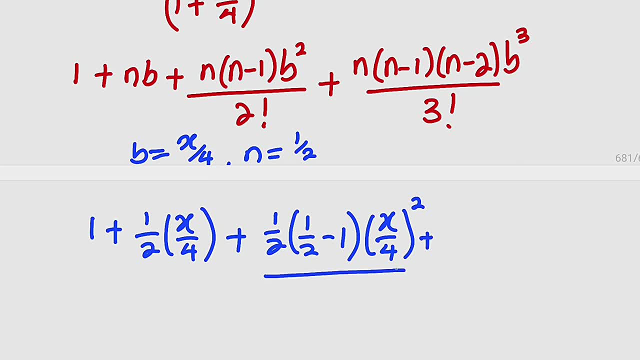 Then the last term will be okay. I have to divide by 2 factorial here. Then the last term will be n, which is 1 divided by 2, multiplied by 1, divided by 2, minus 1.. 1 divided by 2 minus 2.. 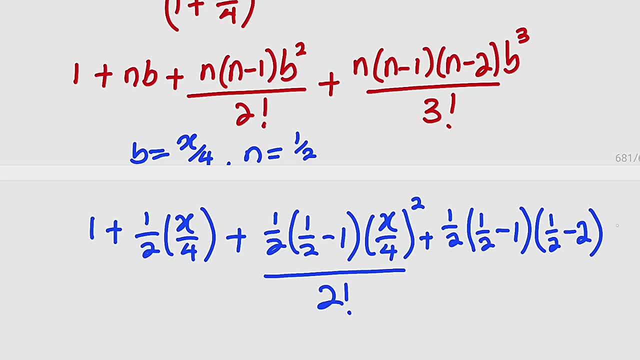 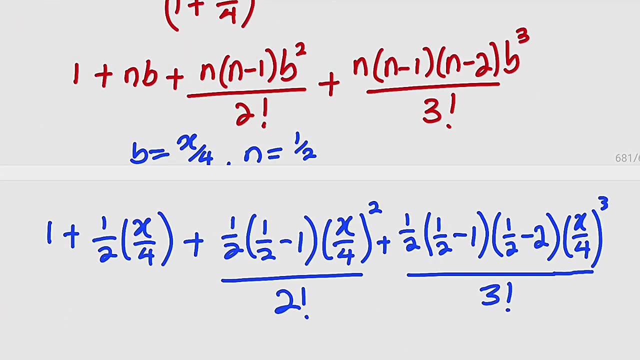 Then b to the power of 3, and b is what x divided by 4.. We have x divided by 4 to the power of 3.. We divide by 3, factorial. Let me shift it to the other side. All right, let us simplify and get our final answer. 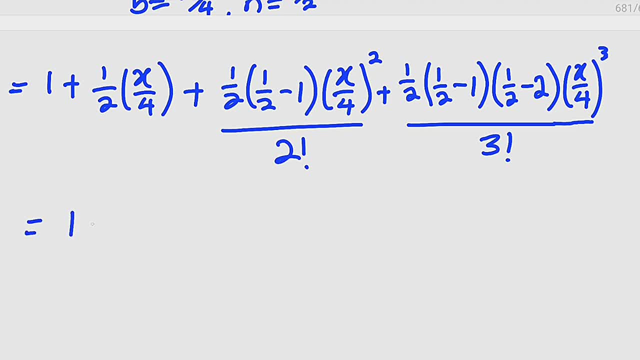 We have this to be equal to 1 plus x divided by 8, right, x divided by 8.. Or you can simply write it as 1 divided by 8 times x. This is plus, or I will get minus because of this. 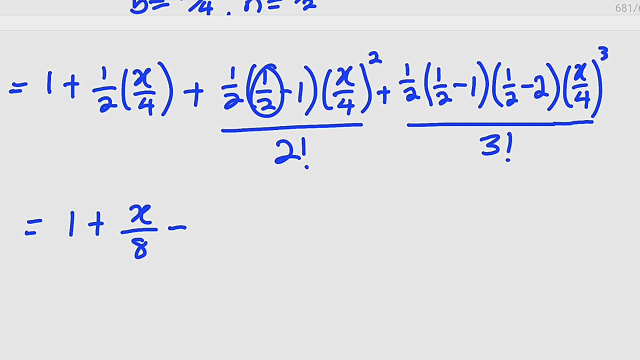 1 over 2 minus 1 is negative 1 over 2.. If you multiply it by this, you get negative 1 over 4.. So we have negative 1 over 4 here. If you expand this, you are going to get x squared divided by 16, right. 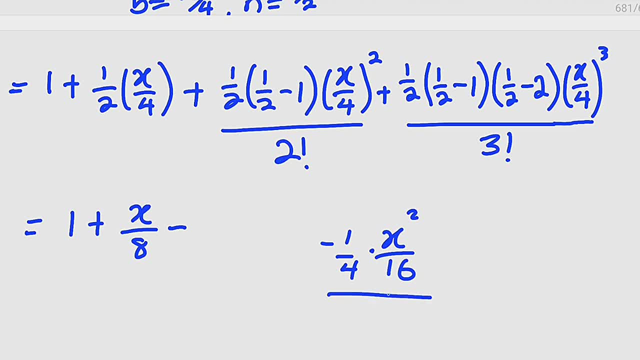 And this 2 factorial is the same thing as what 2.. So this 4 multiplied by 16 will give us 64.. And you know that you have to multiply by this 2.. So you get 128.. So we have negative x squared divided by 128.. 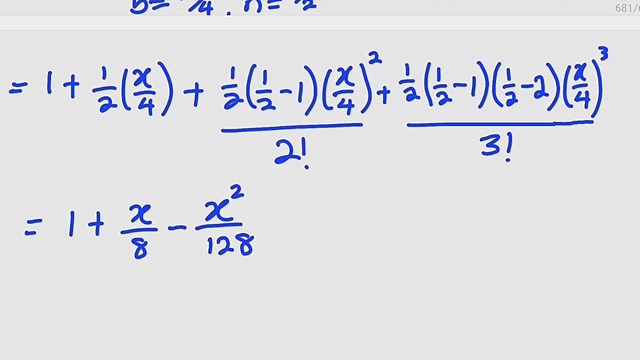 Then we move to the other term. That is the last term. We have 1 over 2 multiplied by negative 1 over 2.. That is half minus 1 is negative 1 over 2.. We multiplied by 1 over 2 minus 2.. 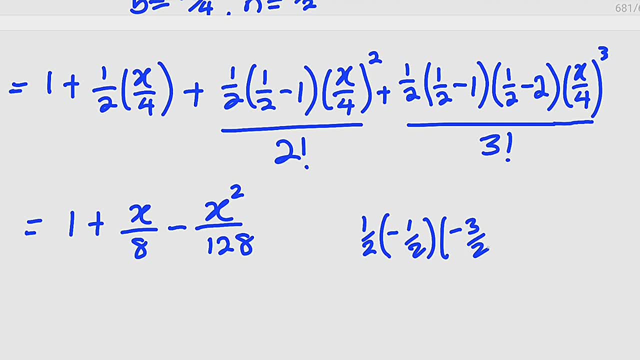 That is negative 3 over 2, right Negative 3 divided by 2.. Then the last one, x over 4, all to the power of 3, will give us x to the power of 3 divided by 64. Because 4 to the power of 3 is 64.. 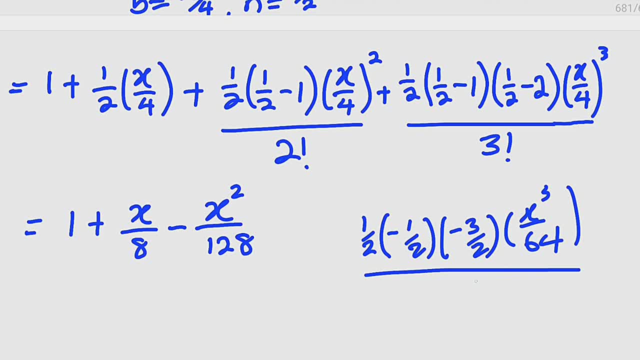 Then we have to divide the whole of this by what? 3 factorial, which is 3 times 2 times 1,, which is 6.. So let us multiply all these denominators together. Let me start from the right-hand side. 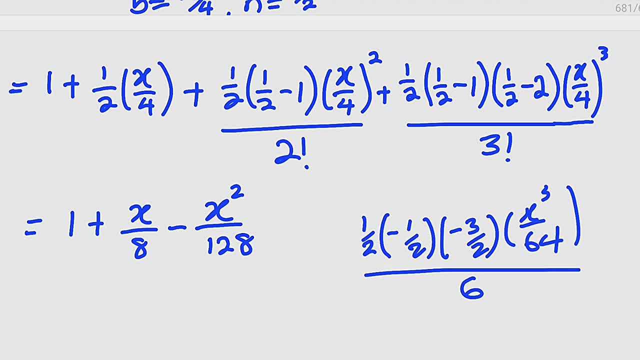 We have 64 times 2,, which is 128,, times also another 2, times another 2, which is 512.. And that 512 will have to be multiplied by this 6. And if you do that, you're going to obtain 3,072.. 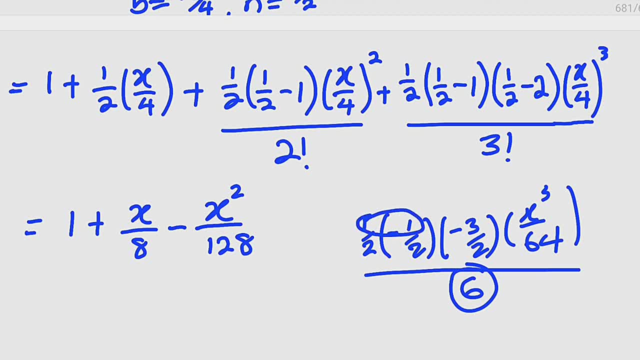 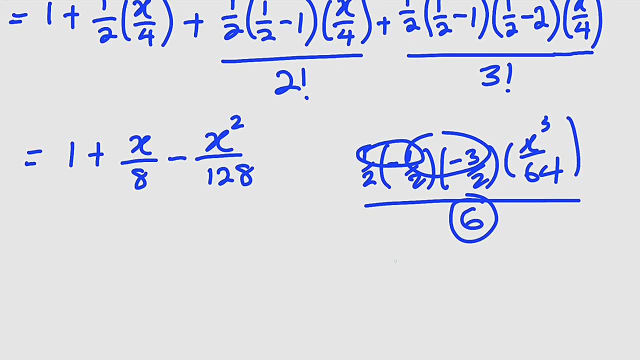 Then to the top, we have 1. times negative, 1, which is negative, 1.. Times negative: 3, which is positive. 3, x to the power of 3.. So all this will be 3x to the power of 3 divided by 3,072.. 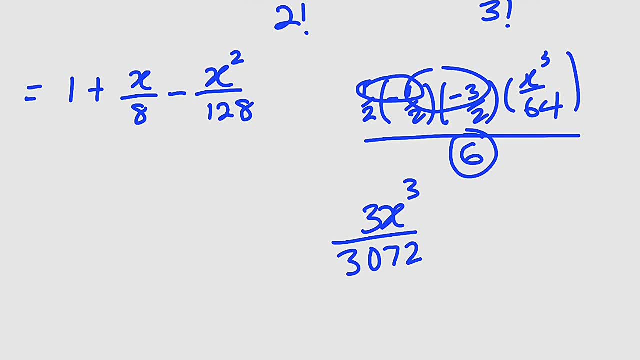 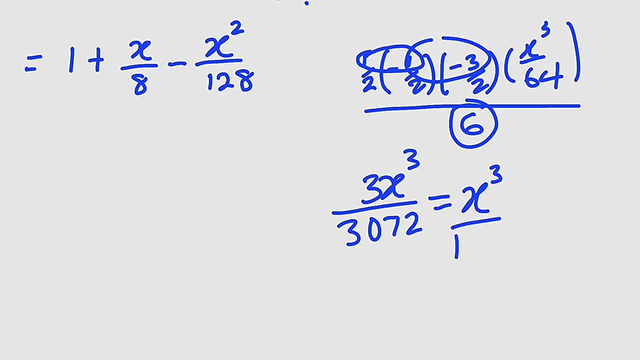 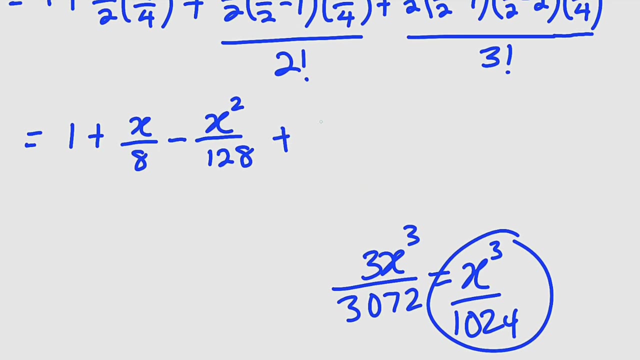 And 3 can go into 3,072, 1,024.. So this, finally, will be x to the power of 3 divided by 1,024.. This is what we need to write as our last step. So we have plus x to the power of 3 divided by 1,024.. 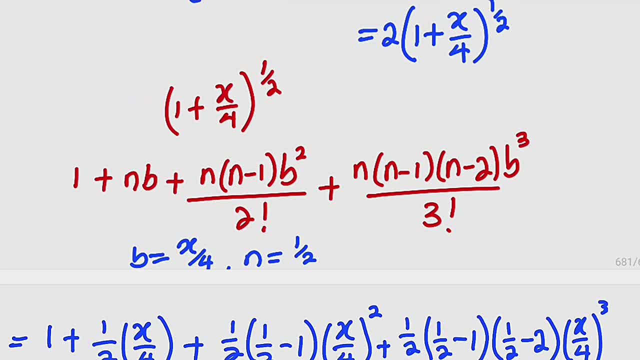 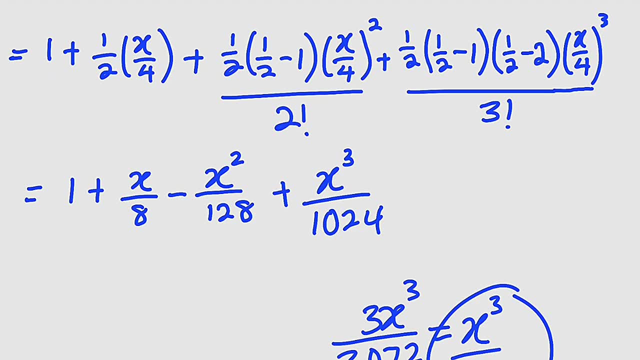 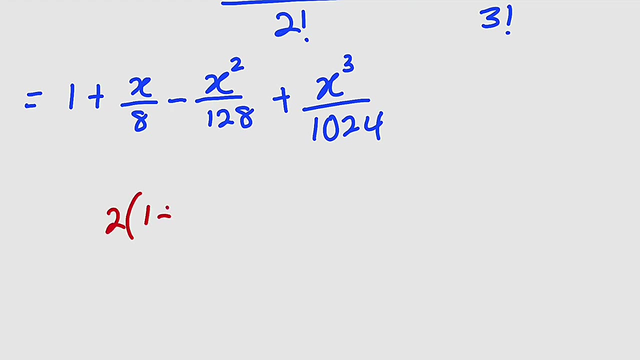 This is the expansion of what 1 plus x divided by 4, to the power of 1 over 2.. That's just the first four times. We have other times, But don't forget to multiply it by these two. So finally, 2 multiplied by 1 plus x divided by 4.. 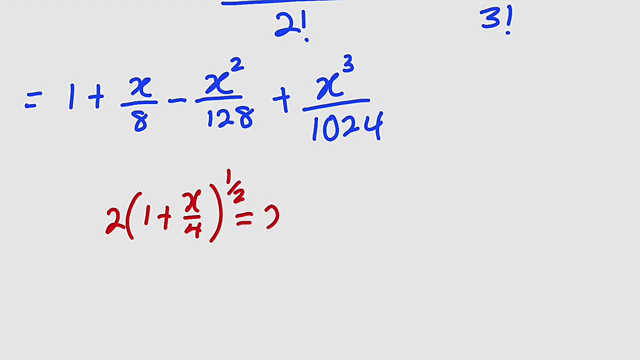 To the power of 1 divided by 2 is nothing but 2 multiplied by the whole of these times 1 plus x divided by 8 minus x, squared divided by 1 to 8 plus x, to the power of 3 divided by 1,024.. 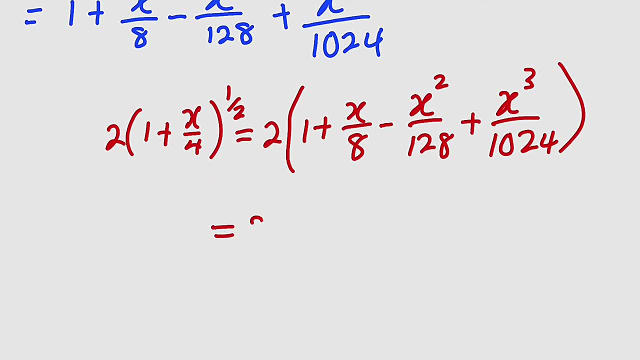 So if you expand this, you have 2 times 1, which is 2.. Then plus 2 can go 4 into 8.. How many times? That is 4 times. So you have x divided by 4 minus 2 into 128. x squared divided by 64 plus x to the power of 3 divided by 2 into 10 is 5.. 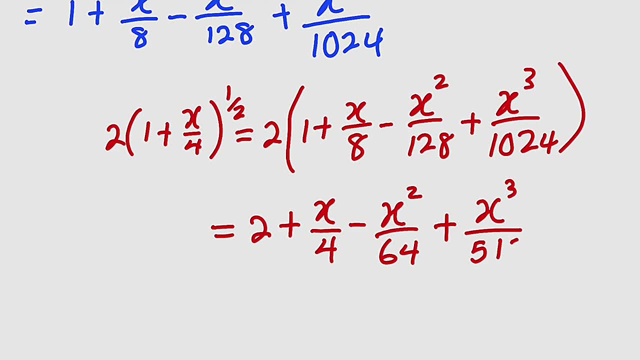 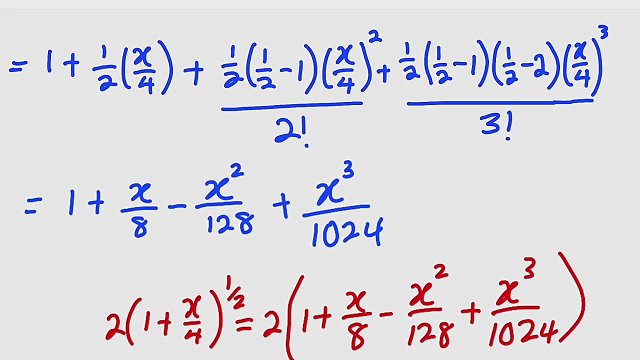 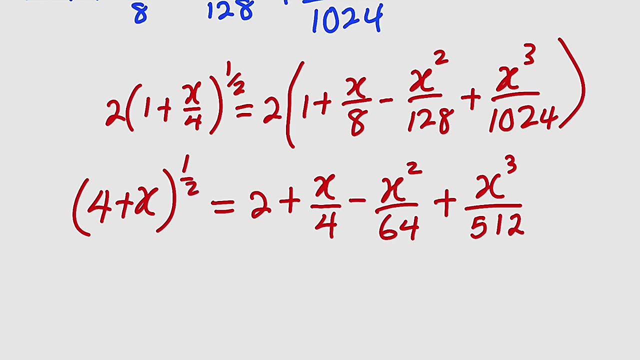 2 into 2 is 1.. 2 into 4 is 2.. So finally, we can say that The whole of this- 4 plus x to the power of 1 over 2- is the same thing as this. 4 plus x to the power of 1 over 2- is nothing but this.